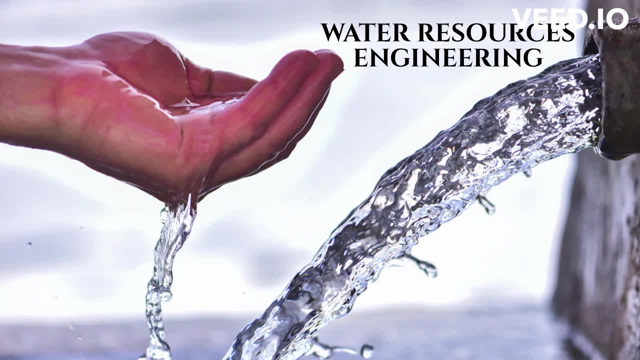 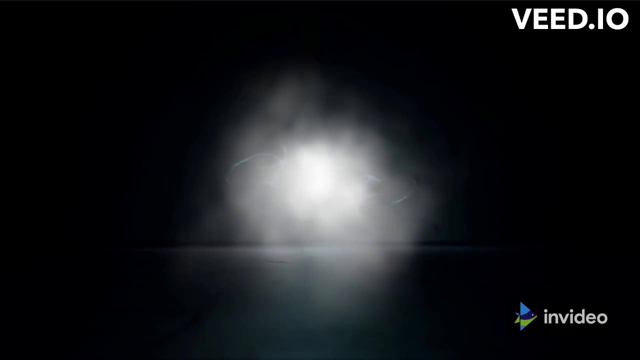 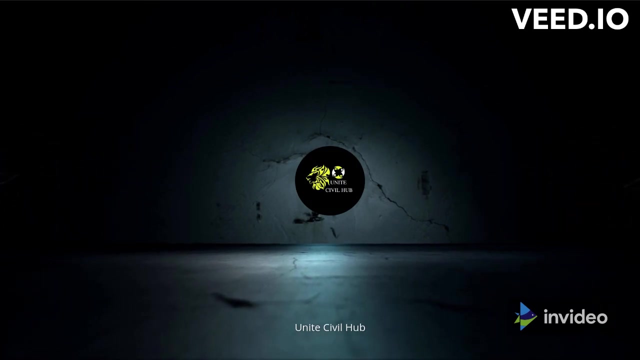 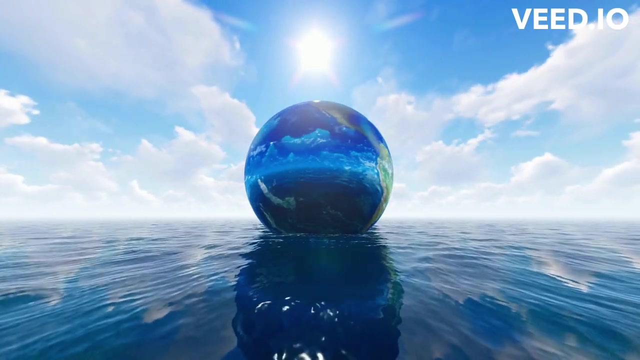 We will also be discussing current and future challenges in water resources engineering, as well as potential solutions to these challenges. Without any further ado, let's move on to the video, Chapter 1. Water Resources Management. The first topic we will be discussing is water resources management. 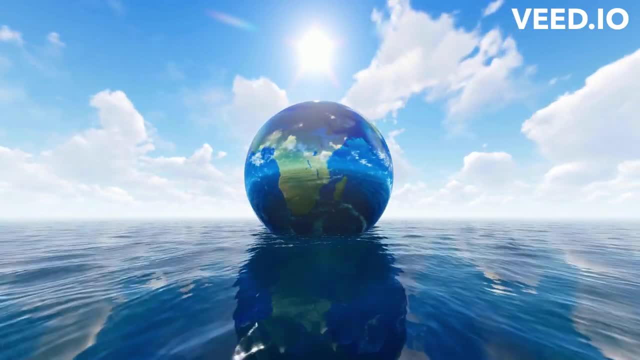 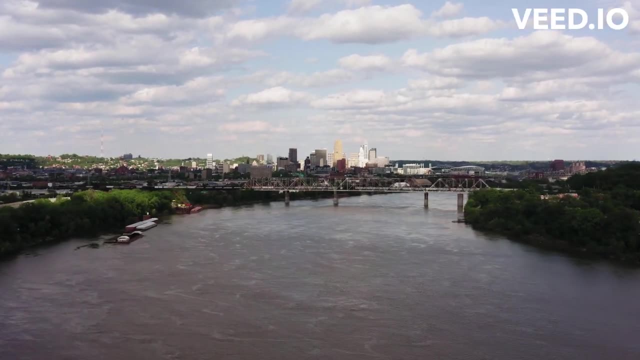 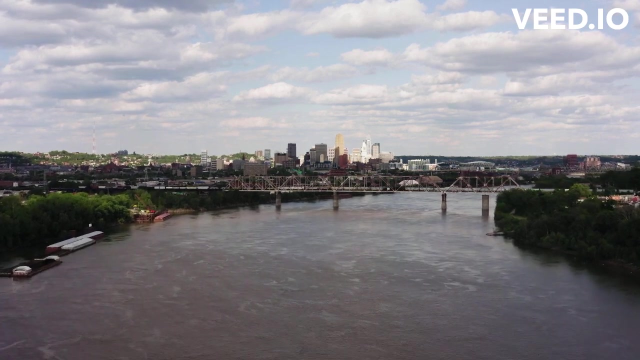 Water resources management refers to the process of planning, developing and maintaining water resources. This includes the management of surface water and groundwater resources, as well as the management of water quality and water supply. One of the key challenges in water resources management is ensuring that there is enough. 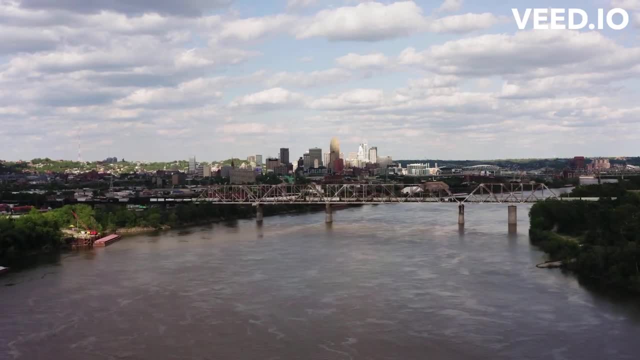 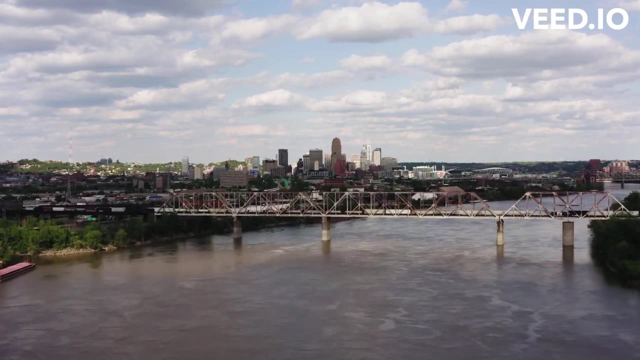 water to meet the needs of a growing population. This includes managing the demand for water as well as managing the supply of water. To meet this challenge, many communities have turned to water conservation and efficiency measures, such as using low-flow water. To achieve this, many communities have turned to water conservation and efficiency measures. 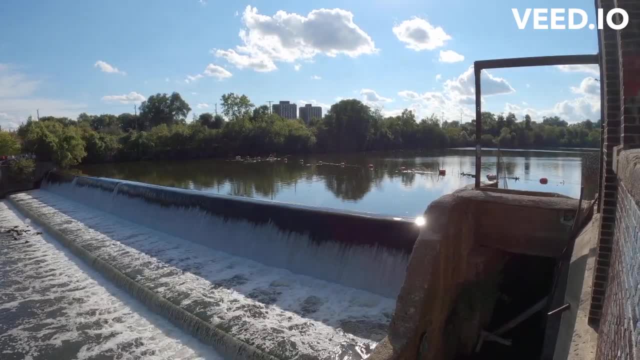 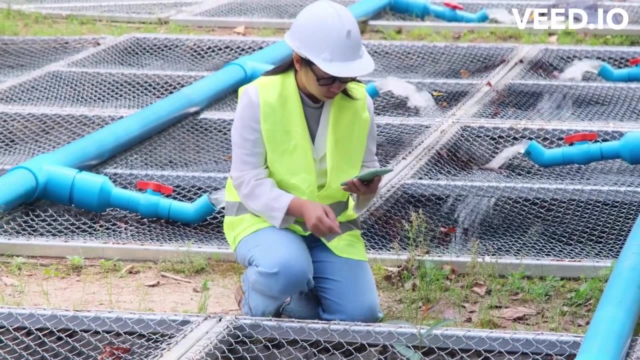 such as using low-flow toilets and showerheads and installing water meters to track water usage. Another challenge in water resources management is managing the quality of water resources. This includes managing the levels of pollutants in the water, as well as managing the effects of climate change on water resources. 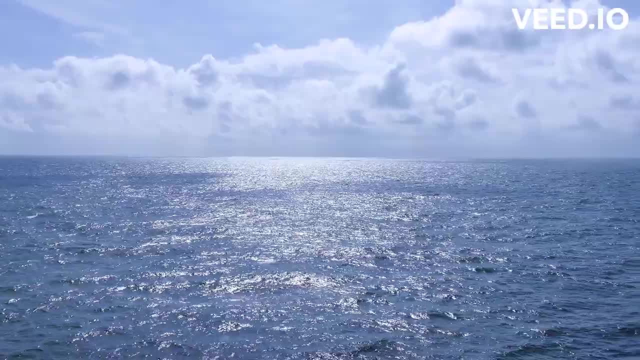 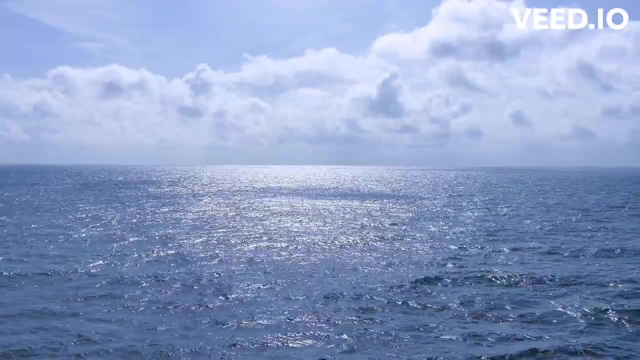 To address these challenges, many communities have implemented regulations to limit the amount of pollutants that can be discharged into water resources and have also implemented measures to reduce greenhouse gas emissions to mitigate the effect of water pollution. To address these challenges, many communities have implemented regulations to limit the amount of 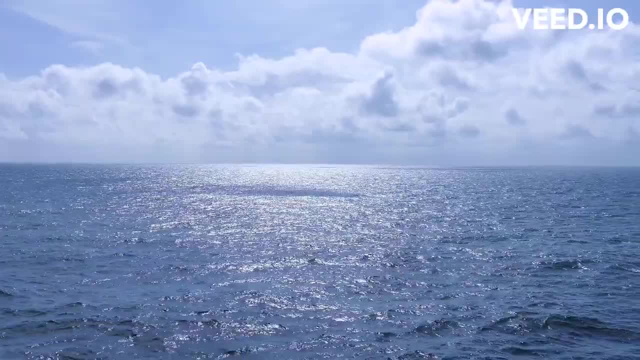 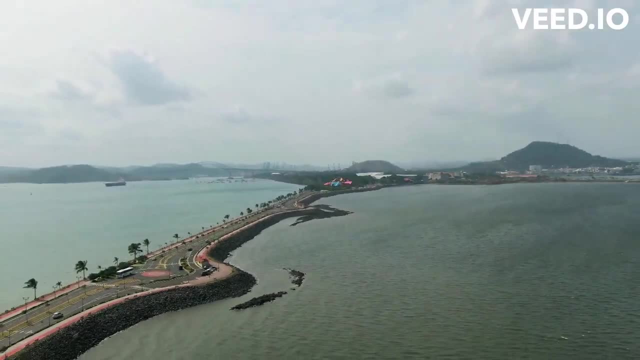 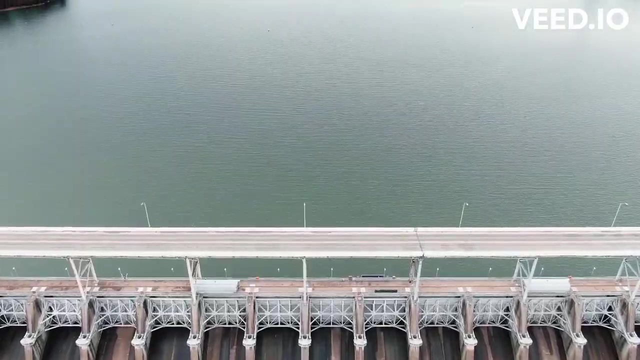 effects of climate change on water resources. Chapter 2. Water Systems Design and Construction. The next topic we will be discussing is water systems design and construction. Water systems design and construction involves the planning, design and construction of water systems, including water supply systems, wastewater treatment systems and stormwater management. 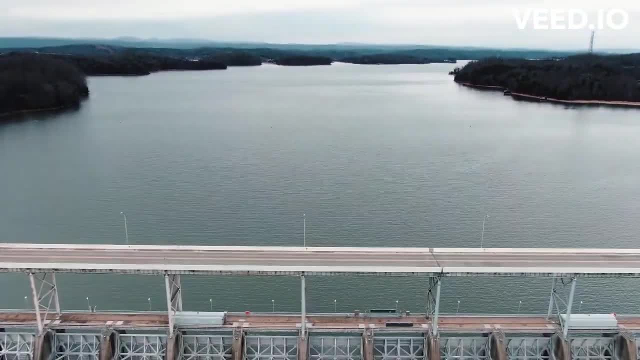 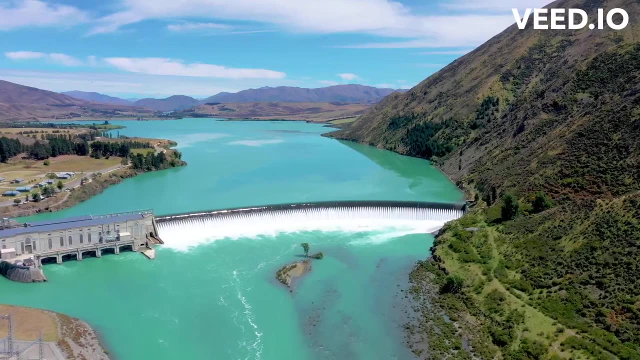 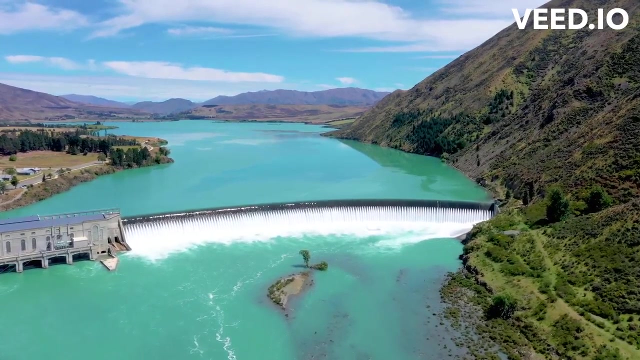 systems. One of the key challenges in water systems design and construction is designing systems that are sustainable and resilient. This includes designing systems that can withstand the effects of climate change, such as sea level rise and increased precipitation, as well as designing systems that are energy efficient and can adapt to changing conditions. Another challenge: 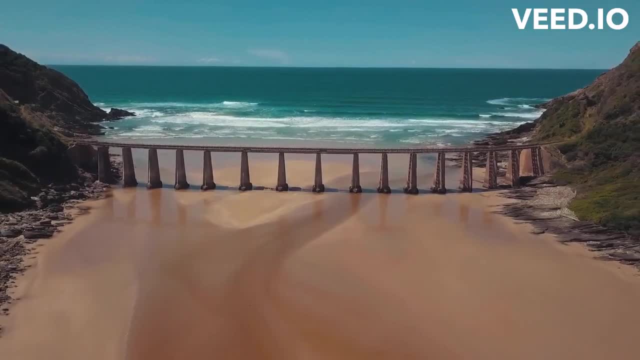 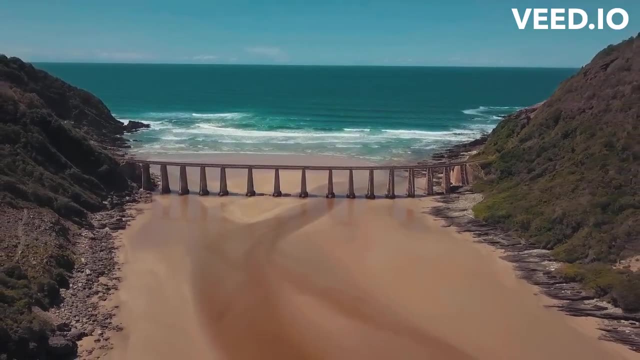 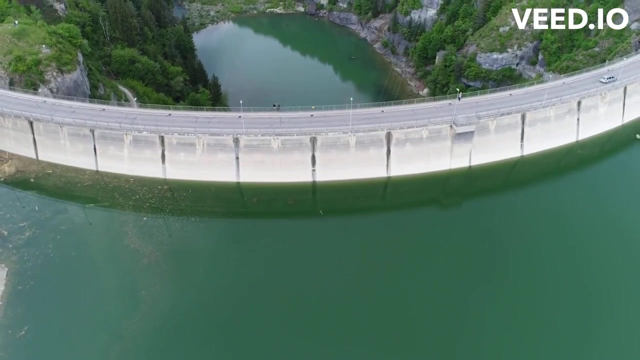 in water systems design and construction is ensuring that water systems are affordable and accessible to all members of society. This includes designing systems that are cost-effective and that can be easily maintained and operated, as well as designing systems that are accessible to all members of society, including those with disabilities. 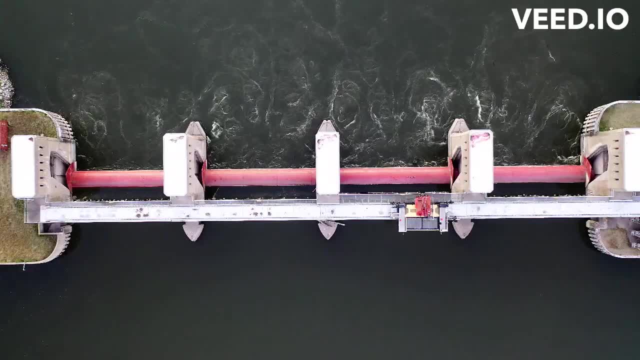 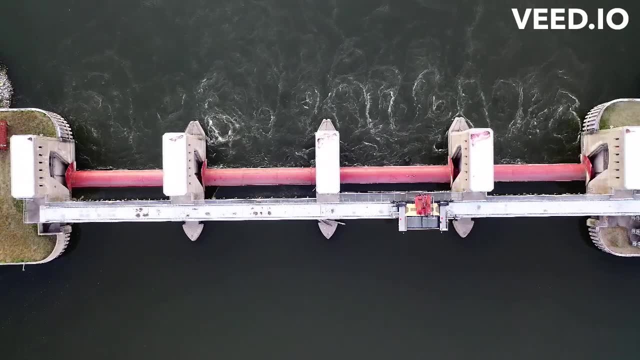 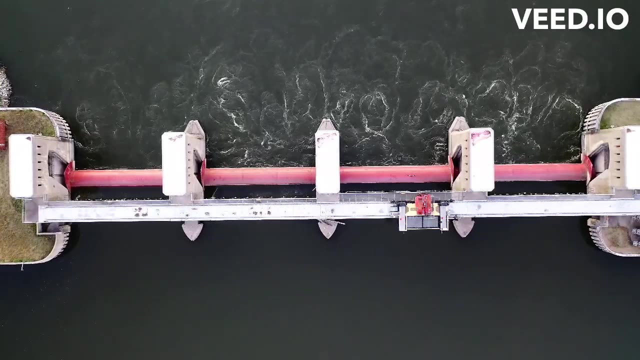 Chapter 3. Impact of Human Activities on Water Resources. The next topic we will be discussing is the impact of human activities on water resources. Human activities, such as population growth, urbanization and industrialization, have a significant impact on water resources. One of the key challenges in addressing the 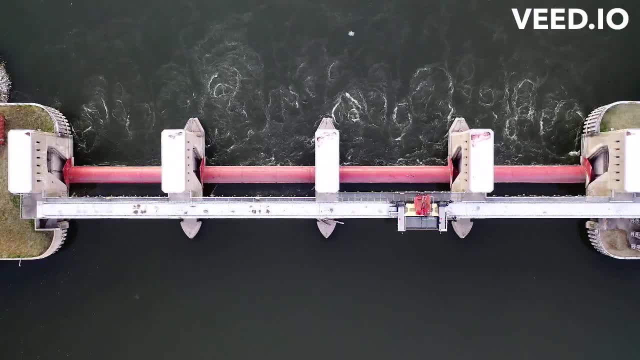 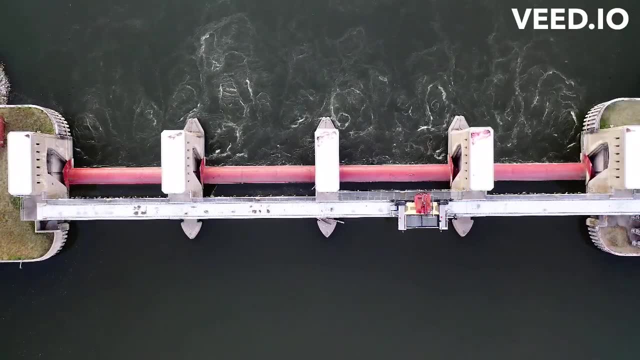 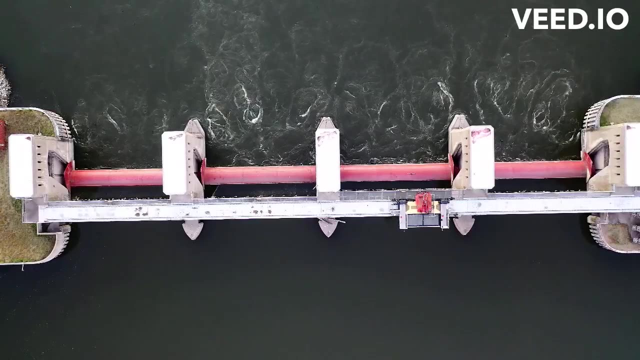 impact of human activities on water resources is the impact of human activities on water resources. This includes managing the effects of urbanization on water resources. This includes managing the effects of increased runoff and pollution, as well as managing the effects of sea level rise and coastal erosion. To address these challenges, many communities have implemented measures such 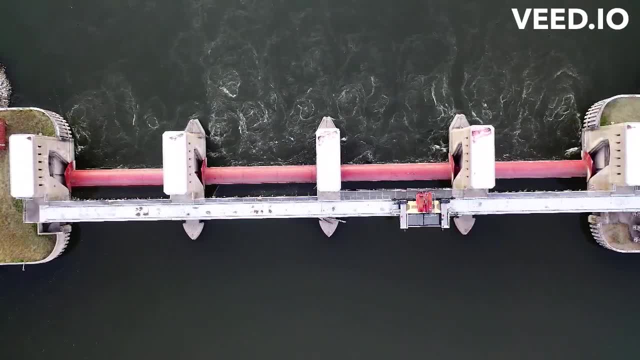 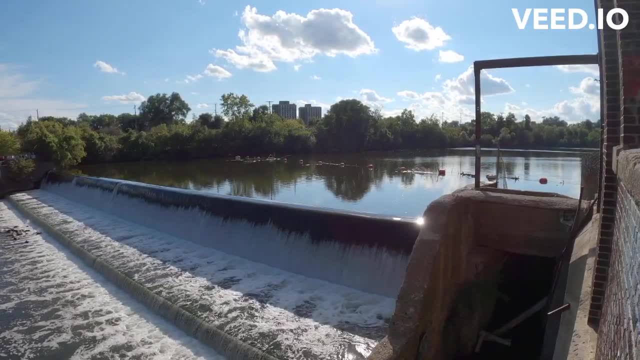 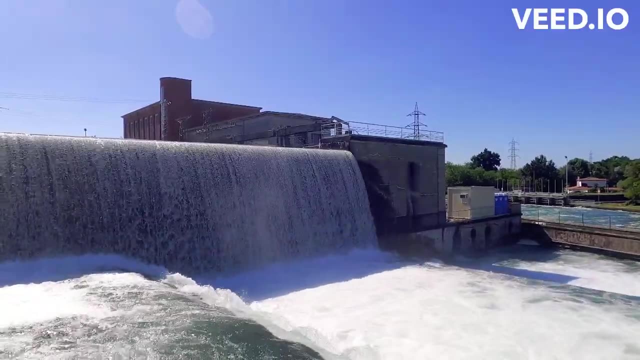 as green infrastructure, which uses natural elements such as trees and vegetation to manage stormwater and reduce runoff. Another challenge in addressing the impact of human activities on water resources is managing the effects of industrialization on water resources. This includes managing the effects of pollutants and waste products. 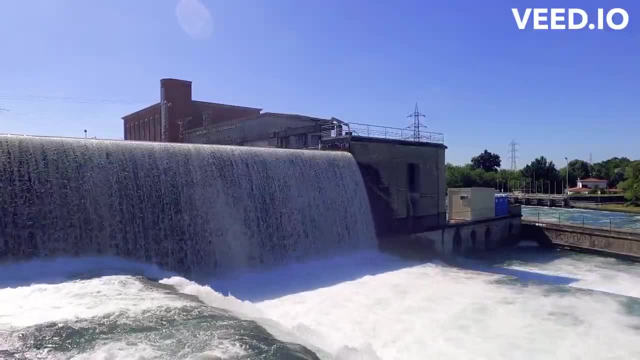 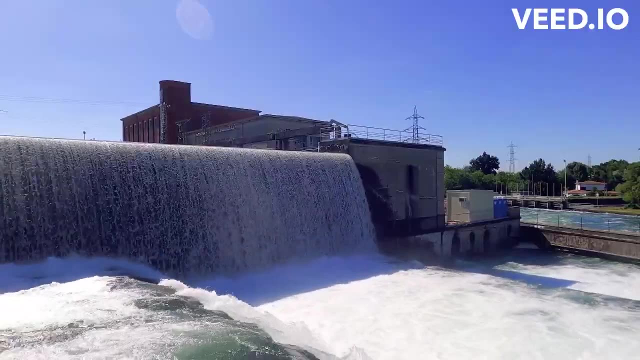 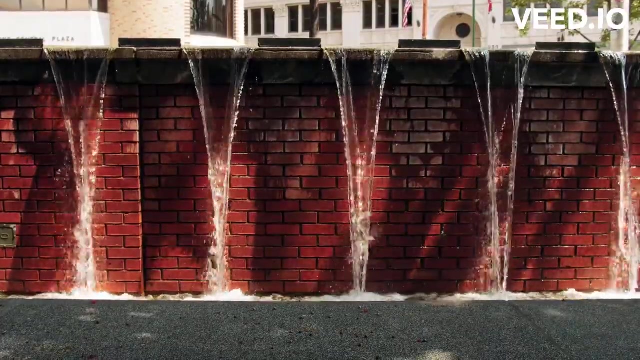 as well as managing the effects of water withdrawal and diversion. To address these challenges, many communities have implemented regulations to limit the amount of pollutants that can be discharged into water resources and have also implemented measures to reduce the amount of water that is withdrawn and diverted. Chapter 4. Current and Future Challenges. 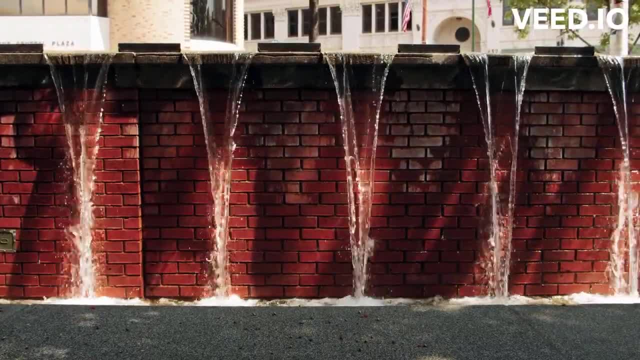 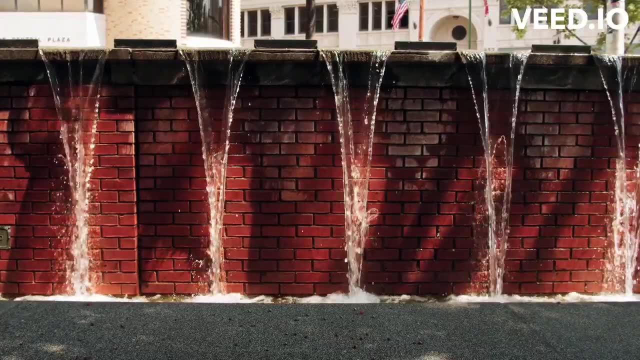 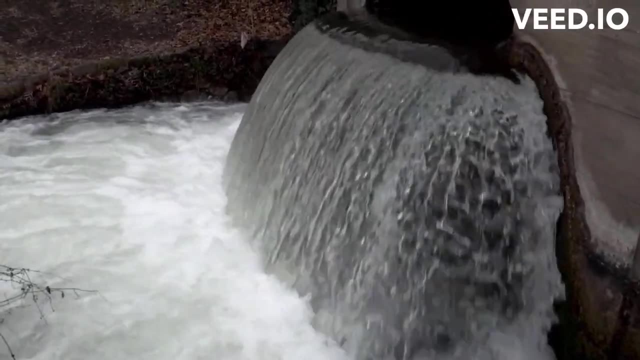 in Water Resources Engineering. In this chapter, we will be discussing the current and future challenges in water resources engineering. These challenges include climate change, population growth, urbanization and industrialization, as well as the increased demand for water and the need to protect and conserve water resources. 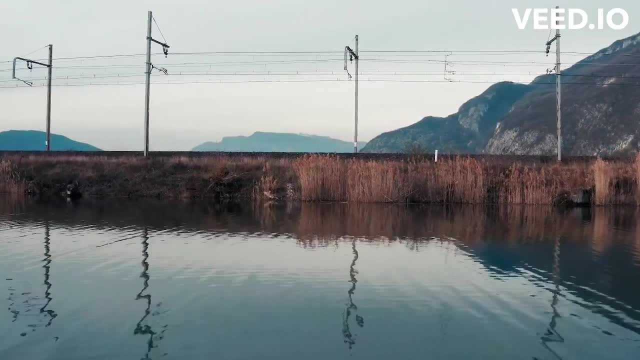 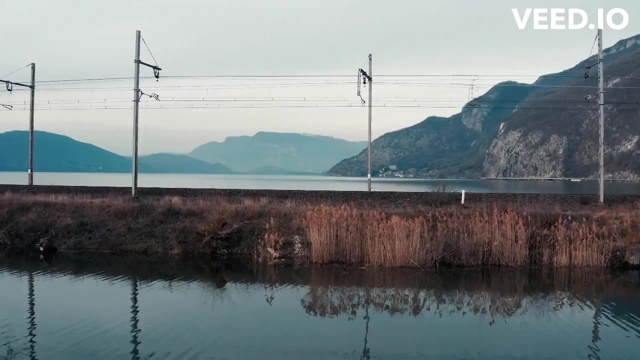 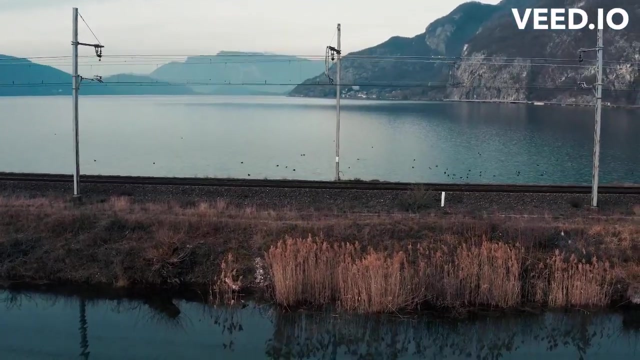 Climate change is a major challenge for water resources engineering. The effects of climate change, such as sea level rise, increased precipitation and droughts, can have a significant impact on water resources. To address these challenges, many communities are implementing measures such as green infrastructure.